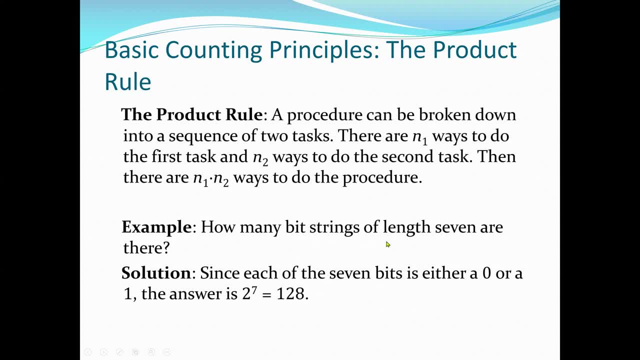 And another example given here is: how many bit strings of length 7 are there? How many bit strings of length 7 are there? Now we know the bit will be only 0 and 1.. So the bits are 2, 0, 1. And the length is 7.. So this means our solution will be 2 to the power. 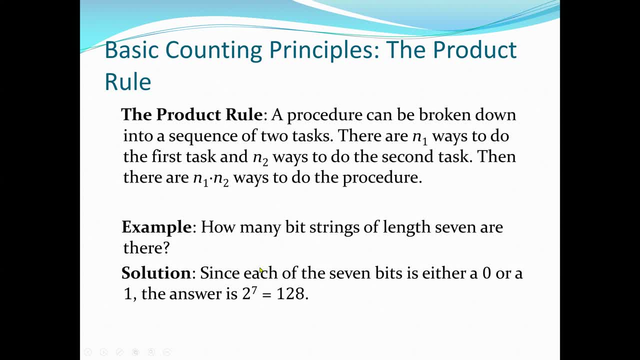 7,, which is the same as saying we have a string which is only 2 bits- 0 and 1, and the length is 7.. So, which means I have to, How many bits we have now will be 2 times 2 times 2, 7 times. 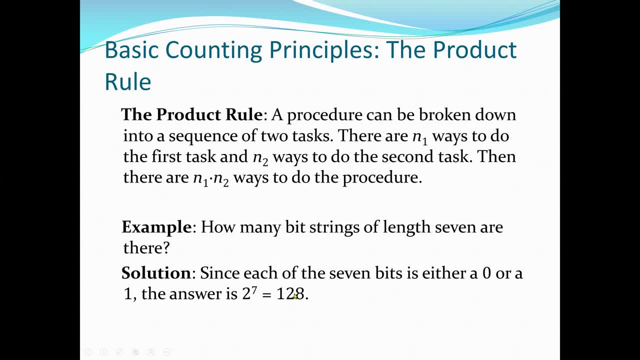 So we write 2 to the power 7,, which is 1 and 28.. So this is again a product rule. How many bit strings of length 7 are there? The bits are only 2,, 0, and 1, and the length is 7.. 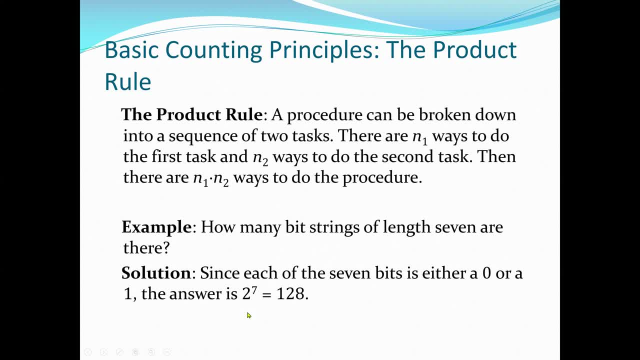 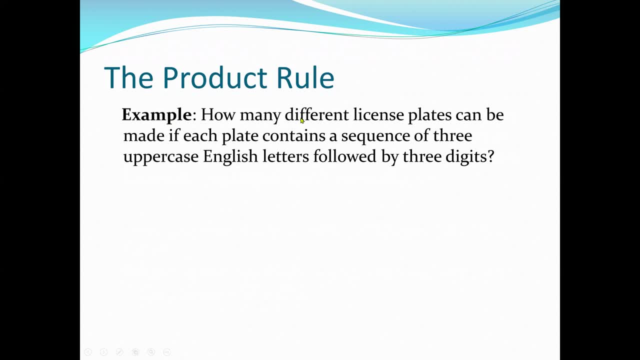 So it will be 2 times, 2 times 2, 7 times, which is 2 to the power 7.. Another example: here we say how many different LanSense plates can be made if each print contains a sequence of three uppercase English letters followed by three. 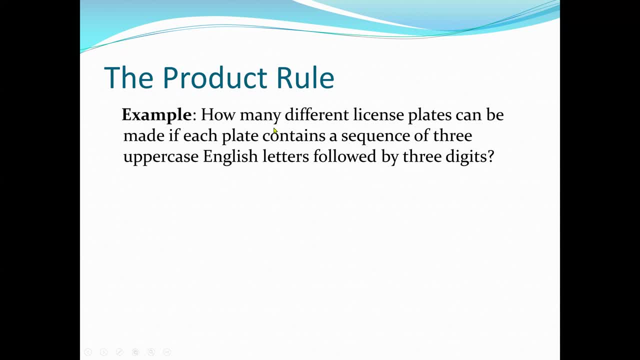 digits. This is also a product rule. So since here our Lancet print may have some amount of three uppercase letters, we know we have 26 letters in English. English letters is 26. So uppercase is 26.. Now the first one. when we are getting the first letter, we have 26. 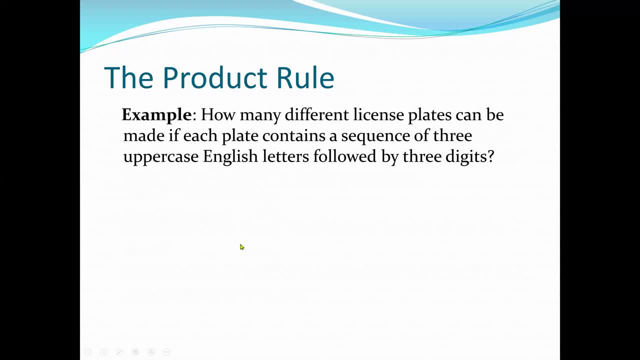 possible Now, if is we to replacement, then we're going to get 26 second, 26 third, But again, We cannot have the same number twice. then that means the first will be 26,, the second will be 25,, the third will be 24.. 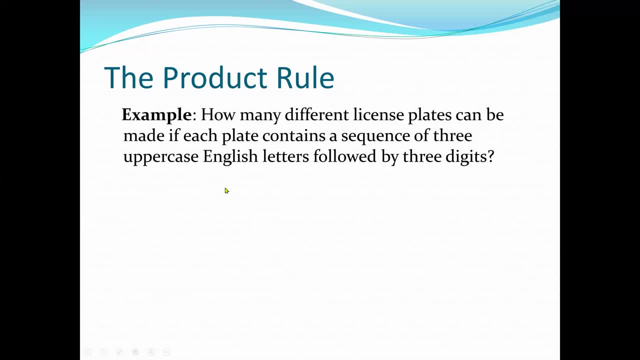 But if we can have this one print twice or three times for the sequence, then it will be 26 times 26 times 26.. Now this is also followed by three digits. So we know, here we are talking about decimal digits. then we have 10, from zero to nine. 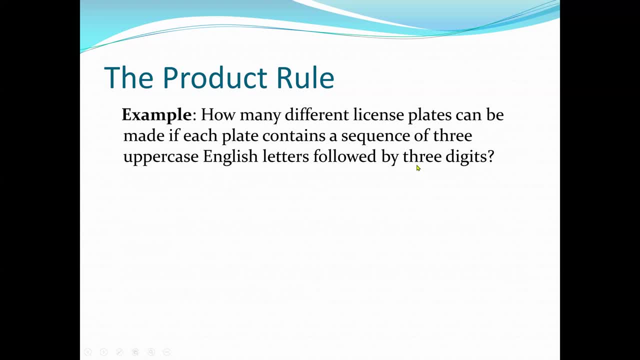 So we can either write 10 times 10 times 10, if possible. unless we say that we cannot have the same digit twice, then it will be 10 times nine times eight. So the possible how many different Lancet sprays we can have will be 26 times 26 times. 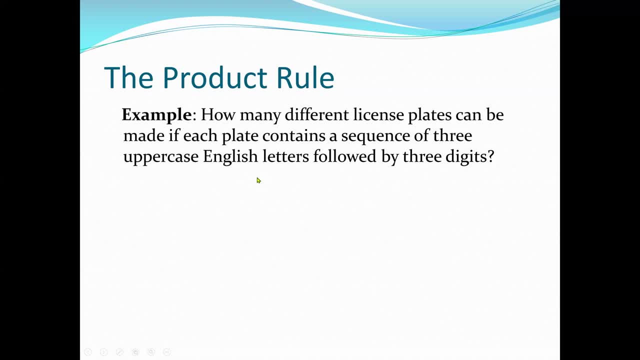 26 times 10 times 10 times 10.. If the letters can repeat itself and also the digits can repeat itself, But if they cannot repeat themselves, then it will be 26,, 25, 24, then times 10, nine. 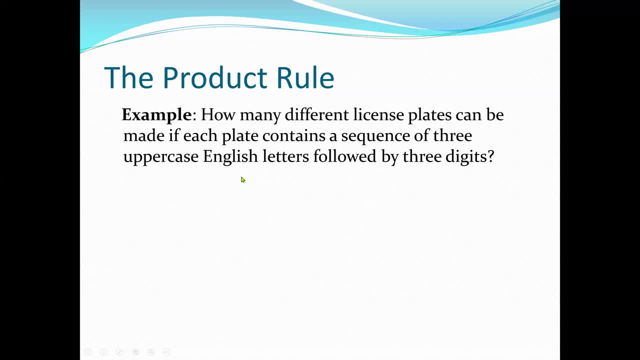 and eight, So it will be 26 times 25 times 24 times 10 times nine times eight. You see that we are reducing it by one one, because when we get the digit, we don't want the digit back again in. So let's see this in this solution. 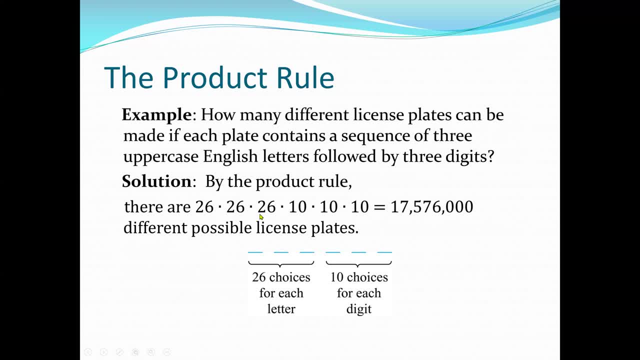 We are saying that We can have three letters at the same time. Let's say, I can have TTT and the digits can be the same digits or different digits. So I can have, let's say, 011 or 111 or 777 or 718, three different digits. 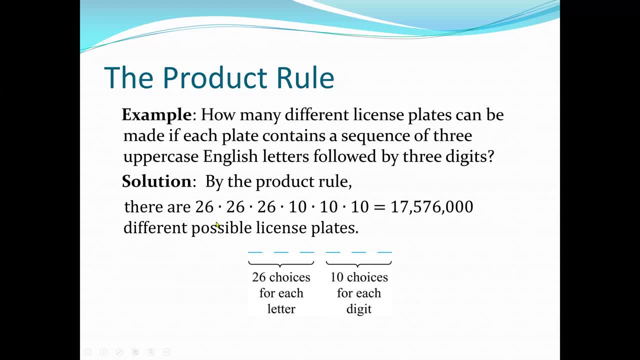 So, as we said, so we, the possible number of Lancet sprays we're going to get will be 26.. The second digit: times 26 times 26, again times 10 times 10.. So we can have three letters at the same time. 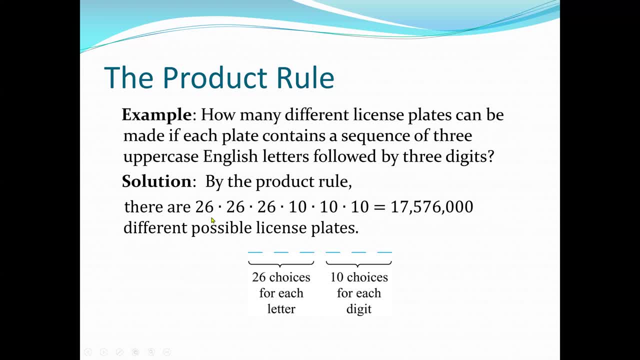 10 times 10 times 10 again. why we choose saying this is because English letters consists of 26 upper cases, So we have option of five in 26 different choice. the same English letter, the second digit, So 26 different choice, 26 now digits consists of 10 digits, from zero to nine. 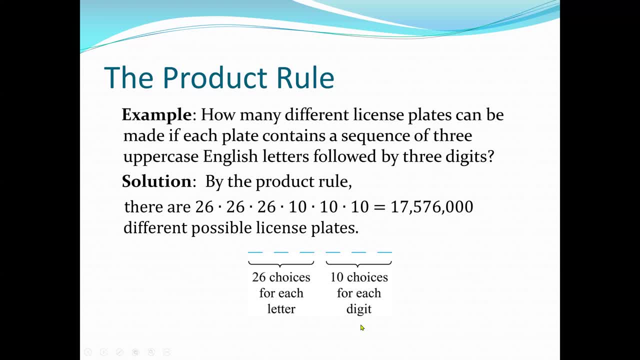 So we have 10,, 10,, 10.. So that will be our total choice. We say 26.. We say 26 choices for each car, each letter, and 10 choices for each digit. So this is again product rule. 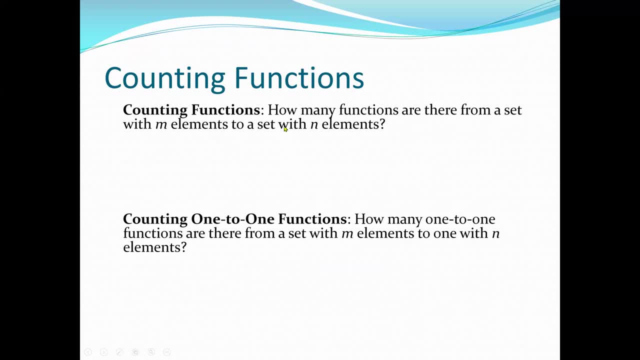 Now, unless we go to the accounting function, we'll say accounting function. Here we are saying: how many functions are there from a set with M element to a set with N elements? So here the solution will be: Yeah, The function represent a choice of one of the N elements of the code domain for each. 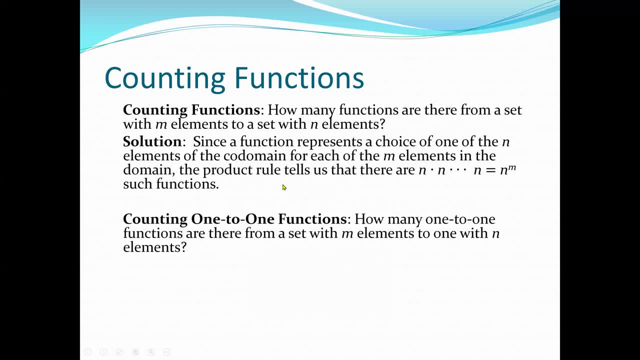 of the N elements in the domain. The product will tell us that they are N times N times N up to M times. So it will be N to the power, M. Again the question: say how many functions are there from a set with M elements? 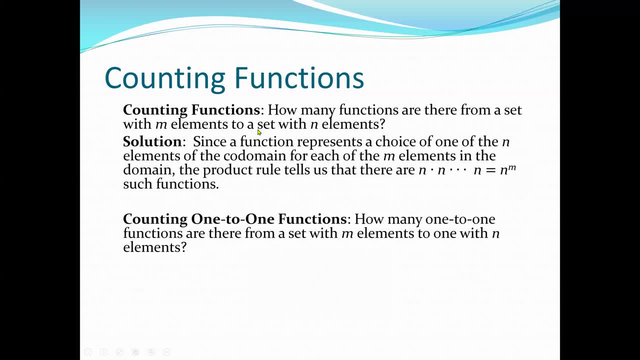 It has M element to a set with N elements. Okay, Okay. So here we are saying: how many functions are there from a set with N elements? It has N elements. So this will give us N up to the M times. So it's N to the power M. So if N is seven and M is 10, then it would be seven times. 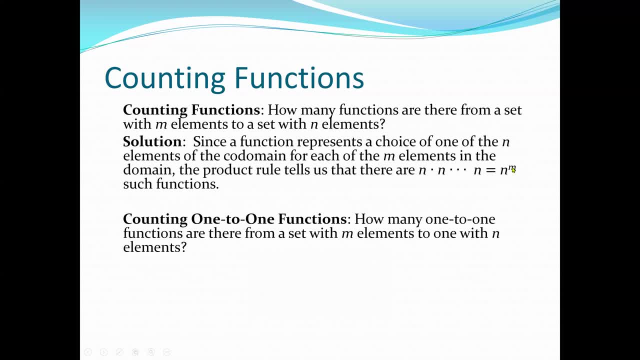 seven, 10 times, which would be seven to the power of 10.. Again, the main thing here is that we said the function It is. It is function since the function represent a choice of one of the n elements of the. 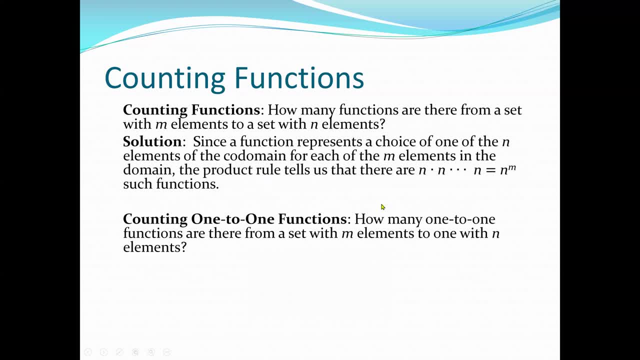 codomain for each of the n elements. so it will be n to the power m. now counting one-to-one functions. here we say how many one-to-one functions are there from a set with m elements to one with n elements. so one-to-one means we are 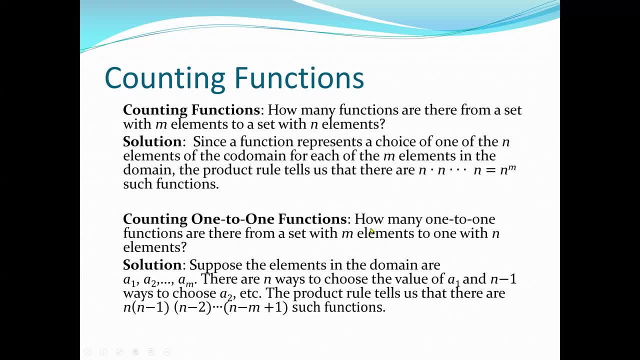 assuming we are assigning how many one-to-one function are there from a set with m elements to one with n elements, so one-to-one m and n. so here we say: suppose the elements in a domain are a1 to am and there are n ways to choose the value of a1 and n-1 ways to choose a2. then we 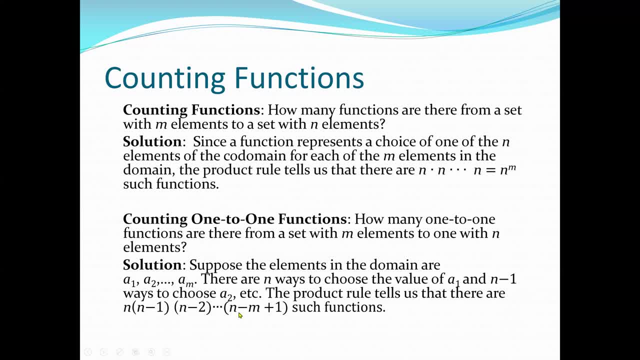 keep going n-2 to choose a3, then the product rule will tell us that there are n times n-1, times n-2, all the way to n-n, plus one such functions, because here we have counting one-to-one function that we enter now at a0. one-to-one is an element of a1, does any? 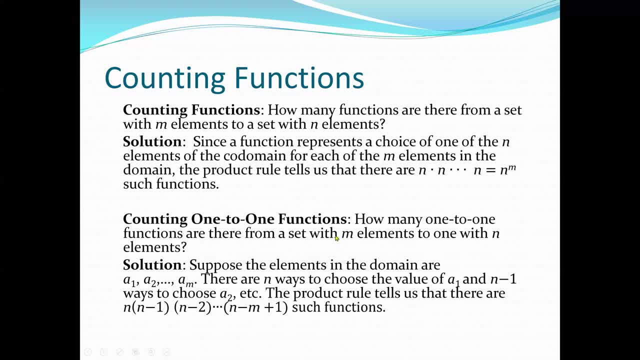 ongoing Arabic class at a0. n- wait is um will keep in this section. there's an element here that's arguing with the program at a2. that's a chain where the, the n of k1, is going to be the creator or an in defence of that variable for a2, ie it will say organic x or mod decimals of koats on b2 instead of a2 and you have to choose n and sometimes that is the celebrates the first part of everything here. 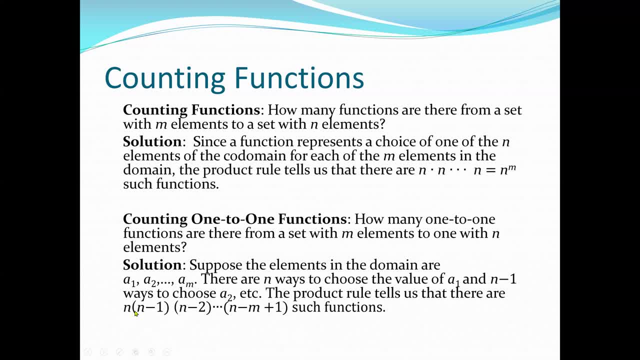 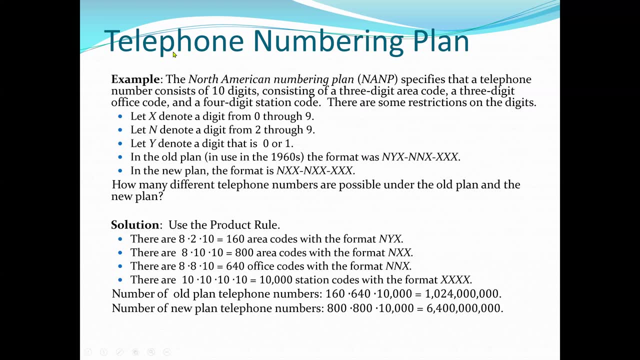 So that means we're going to get n times n minus 1, which is a2, a3, n minus 2, n times n minus 3,, all the way to n minus n plus 1.. So another example is given here by telephone numbering plan. 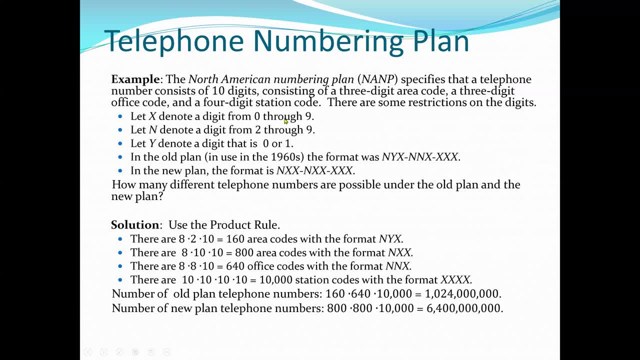 So here we'll come with a replacement of some few rules here. So here we say: in the North American numeric plan it's specified that a telephone number consists of 10 digits. In the North American numeric plan a telephone number consists of 10 digits. 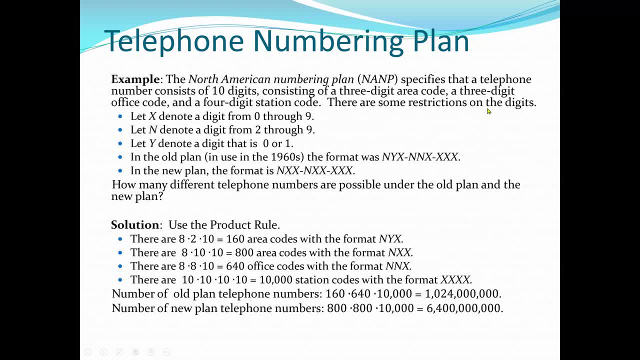 Of a three-digit area code, three-digit office code and then four-digit station code. So there are some restrictions on the digits. So these are the restrictions. We say the X: we donate a digit from 0 through 9.. N- we donate a digit from 2 through 9.. 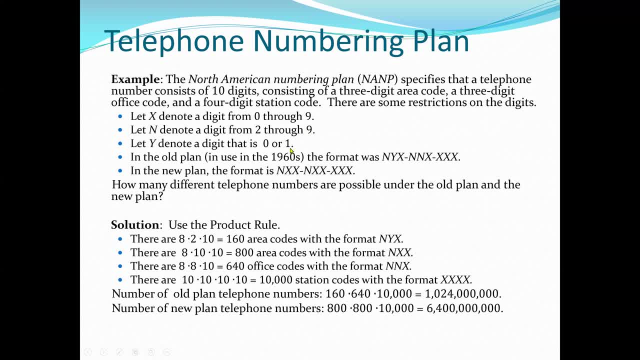 And Y, we donate a digit that is either 0 or 1.. So that's only two options. So now they say in our old plan in use in 1968, the format is NYX, NNX, then XXS. 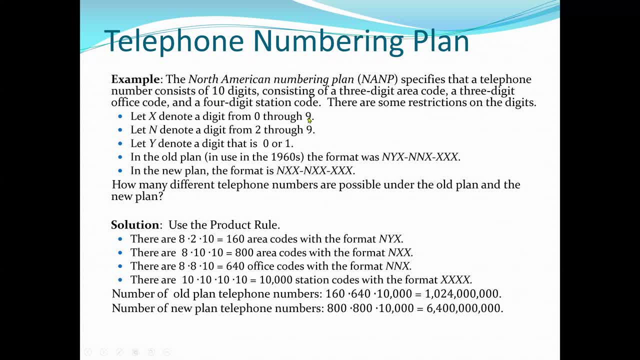 Remember X, So we have from 0 to 9, so 10 options. Then N, we have from 2 through 9.. Then Y, we have 0 or 1.. Now in the new plan we have NXX, NXS, then the last three are also X. 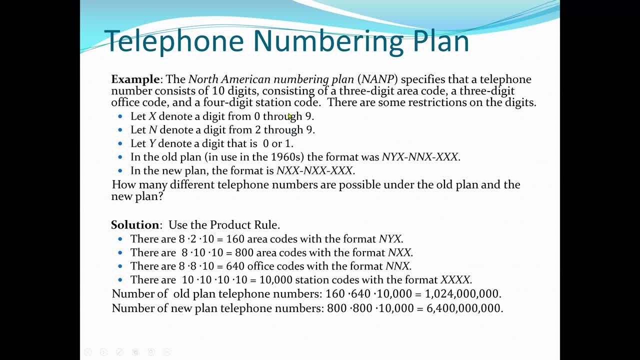 So the solution for this, as we can see- we say the N is 8, because from 2 to 9, we have NXX, From 4 to 9, we have NXX- X is 10.. From 0 to 9,, that's 10 possible digits, 8 possible. 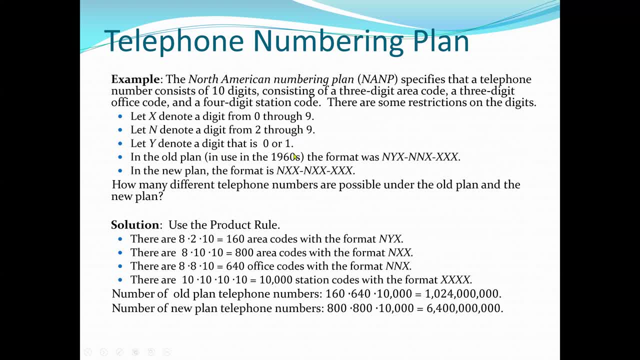 And Y is only two digits, So if I have the format of NXX, then it will be N is what? 8 times 10 times 10.. Then NXS, it is the same thing again: 8 times 10 times 10, then 10 times 10 times 10.. 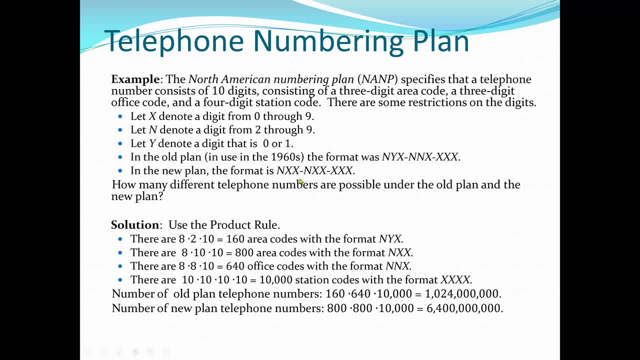 So that will give us the possible combination of telephone number we can get. So here we have the. we start with the old one, first NYX. So we have eight times two times 10, which is 160 for NYX. Now NSX will give us eight times 10 times 10, which is 800. 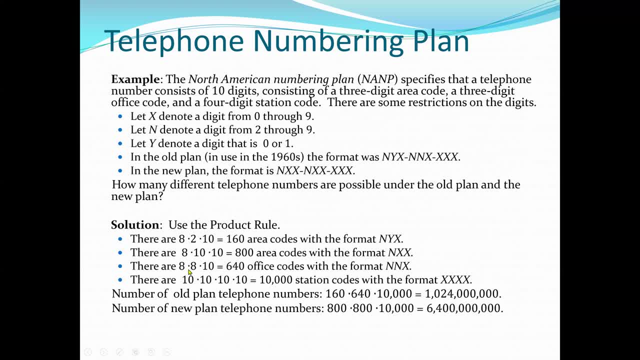 Then we have NNX, which will be eight times eight times 10,, which is 640.. Then we have the Xs throughout. supposed to be 4X is 10 digits of 4X, So it will be 10 times 10 times 10 times 10,, which is 10,000. 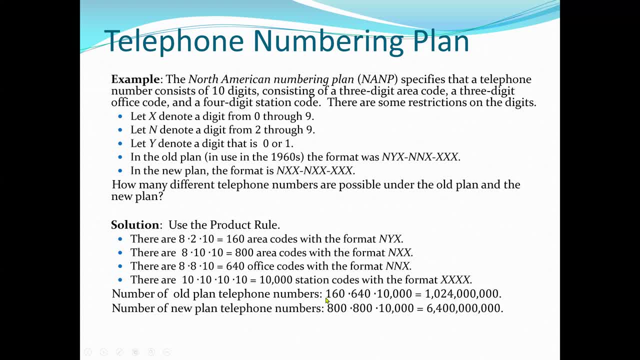 So this means the old plant telephone number system. we have NYX, which is 160 times NNX, which is 640.. Then we have NSX, So it will be 850 times XXX. supposed to be 4X is 10 digits of 4X. 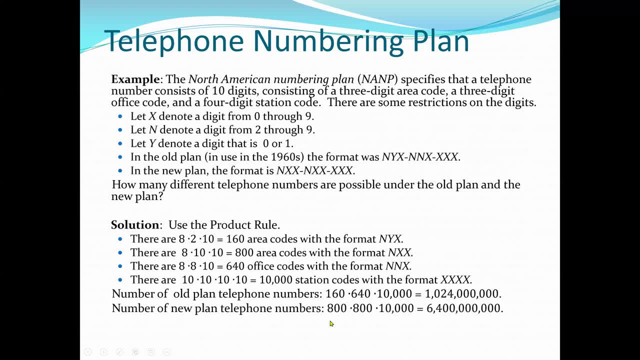 And that's 10,000.. Then the number of new plant. we have NSX, So it will be 800.. NSS is 800.. Eight times 10, times 10.. Then we have NSX, which is we have 800 also. 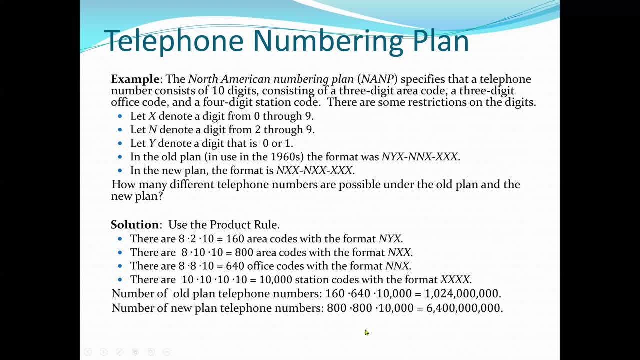 Then SXX for NNX, which is: we have 850.. So we have 800.. Then NNX, which is 850.. Then NNXX, Then NNXX, Which is 600.. So when we multiply the two, the new system will give us over 6 billion, 6.4 billion. 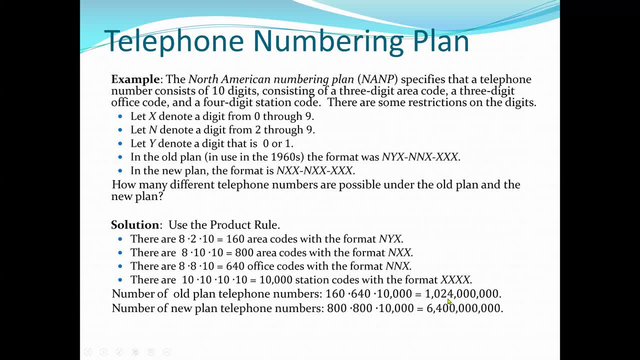 The old system will give us 1.024 billion. So we can see that the rule here tells: determine everything. We said the first digit it should be between zero to nine. The next one, if we have n, it should be a digit only from two to nine. 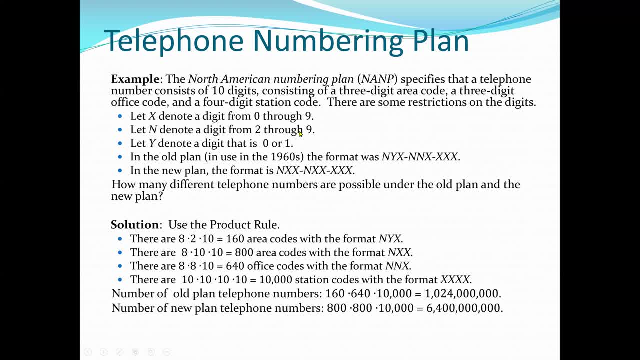 So the possible we can have is eight, And actually the third digit, y, is zero or one. So if I have n? s, x- actually the new plan, they didn't use the y at all. So we have n? s, s, n, s, s, so it will be again, whatever the value of n. excuse me, 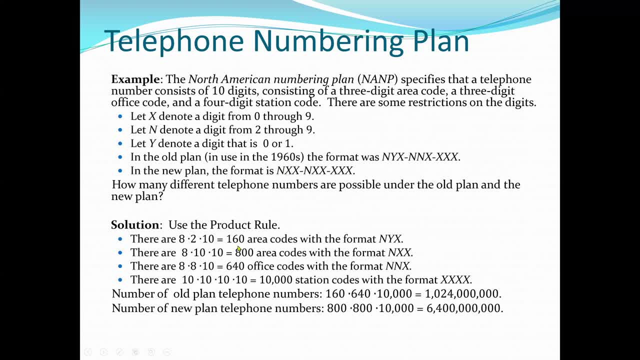 n is eight times two times 10, that's the one. no, sorry, n s s so eight times 10 times 10.. So n s s give me 800 times another 800,. this is supposed to be four x times 10,000.. 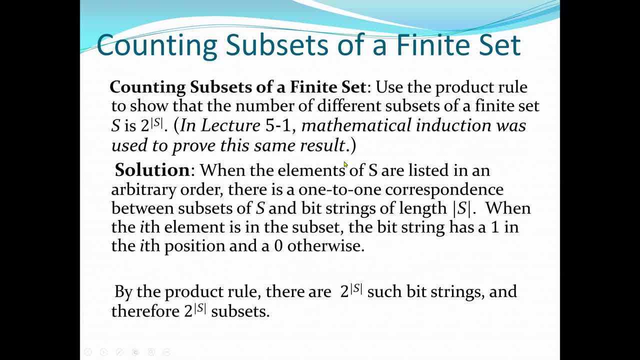 Now the next is counting subset of affinity set. We say counting subset of affinity set. here we are going to use the product rule to show that the number of different subsets of affinity set, which we say s, is two to the power s. actually we again in lecture five, unit five one. we use the mathematical induction. 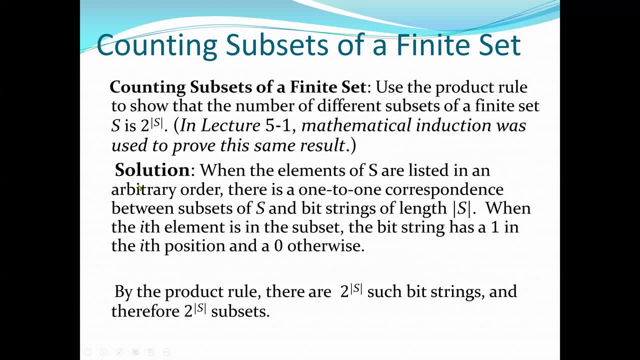 to prove these results. But again, the question says: use the product rule. this time, use the product rule to show that the number of different subsets of affinity set s is two to the power s. Okay, So first, when the elements of s are listed in an arbitrary order, there should be one. 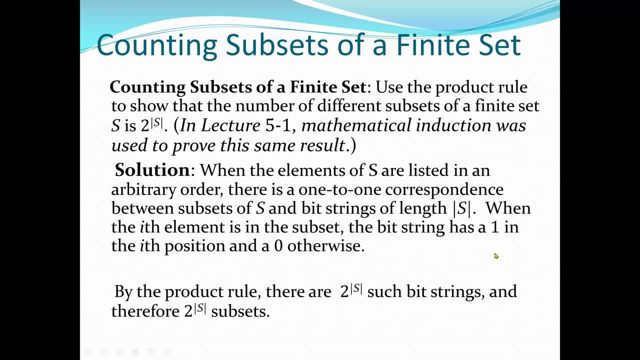 to one correspondence between the subset of s and also the bit strings of x. Now when the if element is in the subset, the bit string has a one in the if position and also a zero otherwise. So in this case by product rule we can say there are two things. 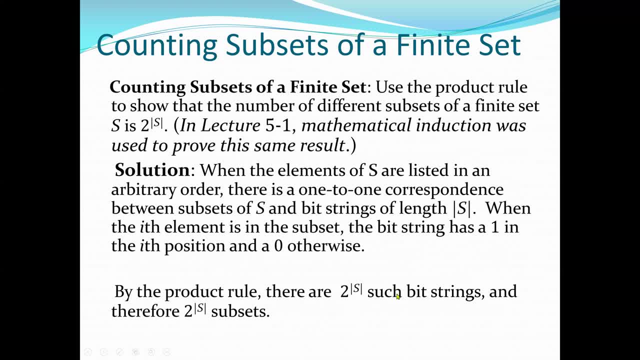 There are two to the power s search bit strings, So therefore two to the power absolute s subsets. Again this very solution. we did this example in using mathematical induction. we can prove this also, But here we are using the product rule to again prove it. 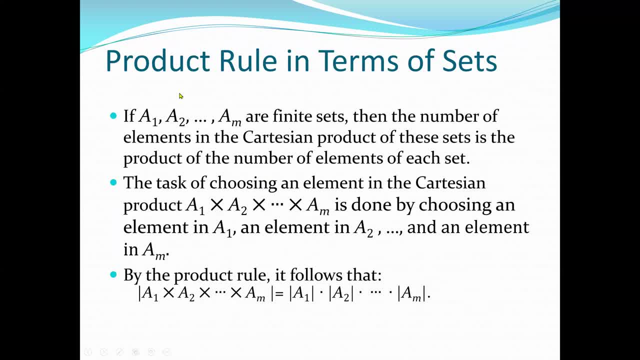 Okay, So, Okay. So a product rule in terms of set. here we say, if we have A1, A2 up to AM as a finite set, then the number of elements in the Cartesian product of this set is again the product of. 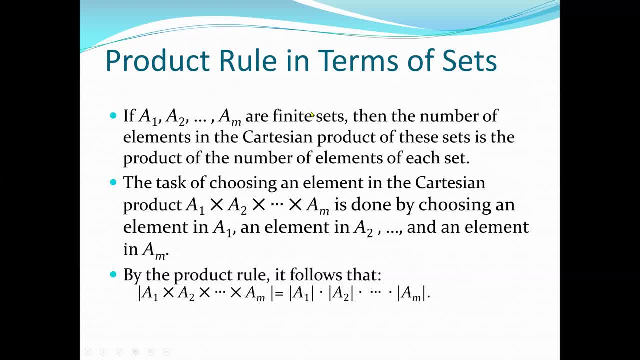 the number of elements of each set We talk about when we're doing the set operations. we talk about Cartesian product. Cartesian product means again, if we have the set of the element, they have to multiply each other and maybe: set here have three elements, set B have four elements. 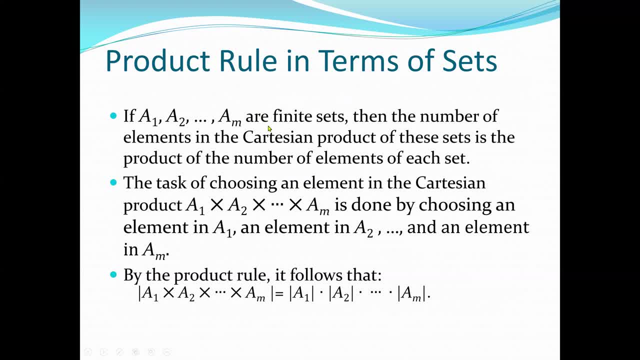 If I multiply the two set together, Cartesian product, I will multiply all the elements by the first set A element, by the set B elements. So here we say, the task of choosing an element in the Cartesian products A1 times A2, all the way to AM, is done by choosing. 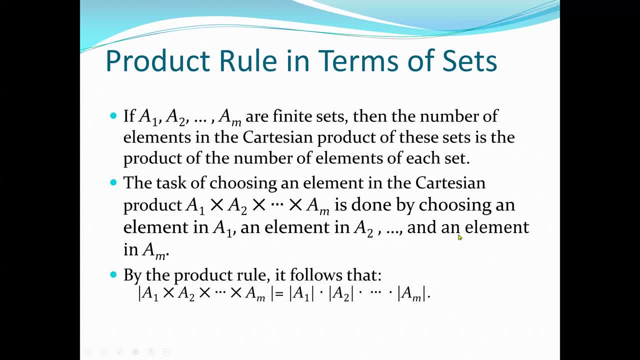 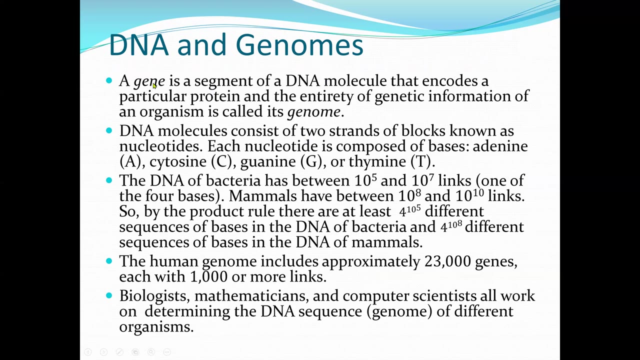 Okay, So by product rule we follow this: A1 times A2 up to AM equal to, again, A1 times A2 up to AM. Also, we have a DNA and genome example here. We know a gene always is a segment of a DNA. 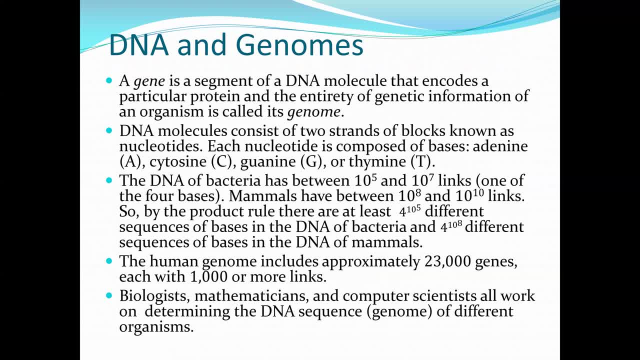 So we may have a DNA molecule out there, We may have a DNA of a thousand, whatever the necrotaurs are, but there will be a segment of the DNA sequence that is a gene. So we'll say a gene is a segment of the DNA molecular that encodes a particular protein. 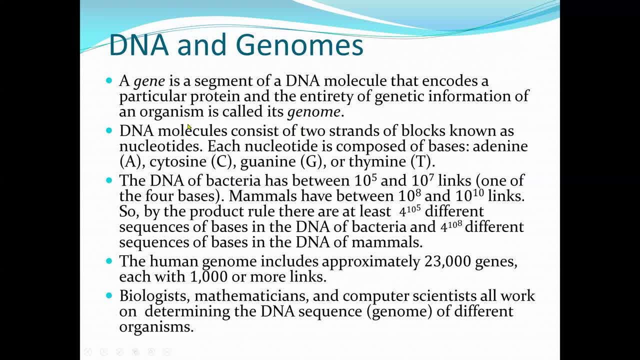 And the entirety of genetic information of our organism is called a genome. The genome will be the component. So the genome will be the component. The genome is a complete DNA sequence of an organism. biological organism for example be a human being or any biological. 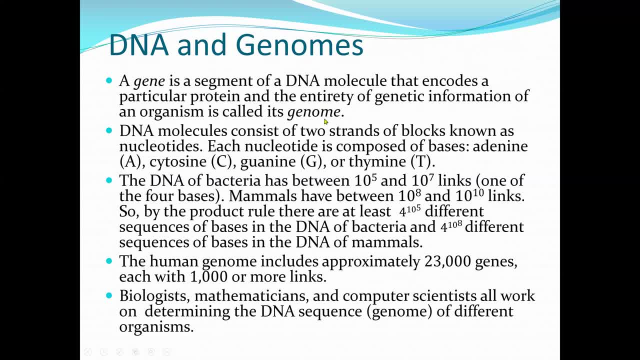 So a genome is a complete DNA of a biological agent. So here we say, the DNA molecules consists of two strands of blocks, known as the necrotites, And each necrotite is composed of bases. The bases is what we call the A, C, T, G, which is the adenine for A, cytosine for C. 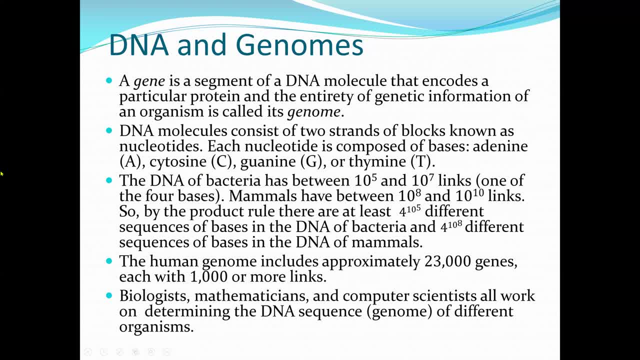 guanine for G and thymine for T. Now a DNA of a bacteria has between 10 to the 5th power to 10 to the 7th power links, Now one of the four bases we see mamas have between 10 to the 10th power links. 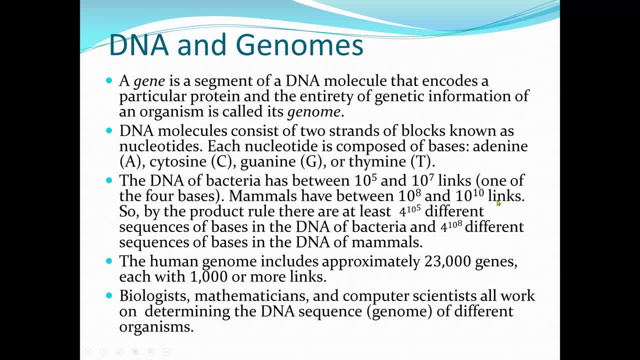 10 to the power 8 and 10 to the power 10 links. so bacterias are between 10 to the power 5 and 10 to the power 7.. so by product rule we can say that they are at least. you see, we are using four. 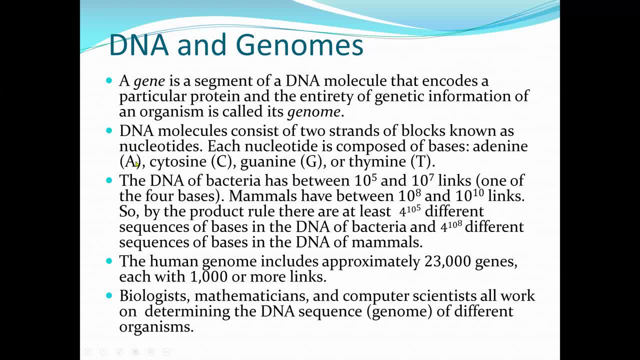 why? because we have the necrotides consists of four, the, the bases are four, so we can say four to the power, 10 to the power fifth. different sequence of bases in the dna of bacteria. because the length of the the bacteria is 10 to the power fifth. start from 10 to the power fifth. 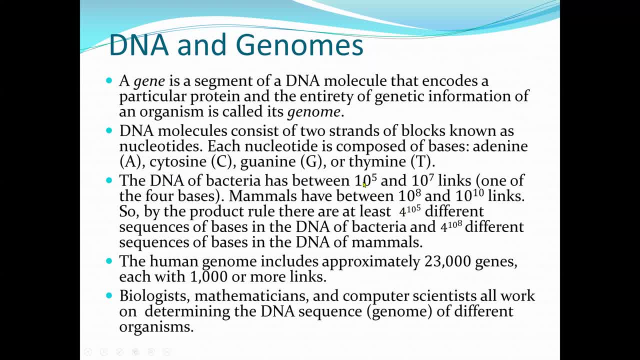 and we know the possible combination sequence we have only for agtc, so it will be four to the power, 10 to the power. fifth, and this will be different form of sequences basis in the dna of a bacteria. now, with the mammals we have 10 to the power eight, so it will be four, 10 to the power. 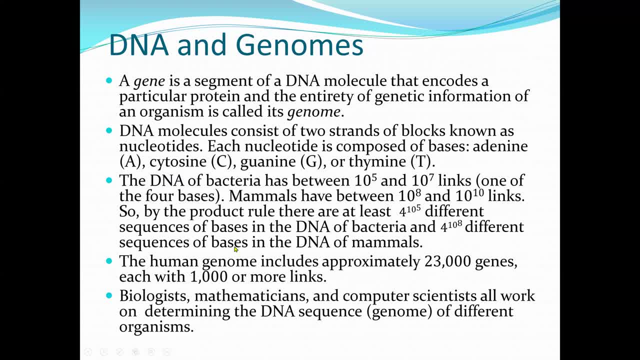 eight different sequence of bases. again, the bases are four, so if the length is 10 to the power eight, they need to be four raised to the power 10 to the 5. 8 is the same as when we are looking for a sequence of a string. we say we need a string string sequence and we say the strings have only. 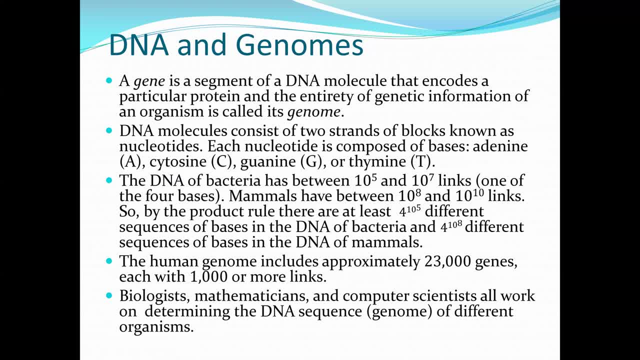 two bits zero and one. the length of the string is seven, so the possible again will be two to the power seven. now, human genome include approximately 23 000 genes, each with thousand or more links, and here the biologists, mathematicians, computer scientists are all working together to determine. 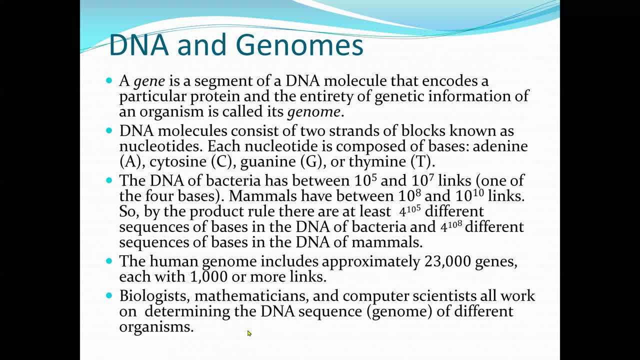 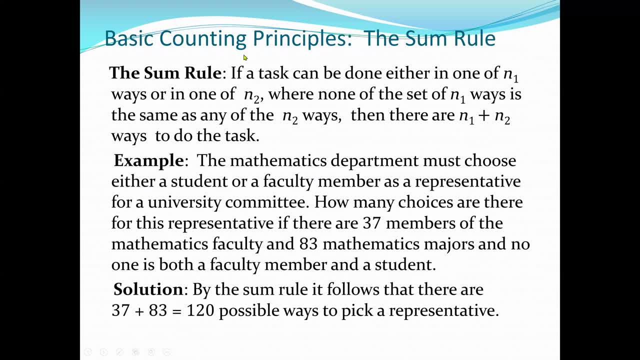 the dna sequence genome of different organisms. the dna is a number of pure cells and there are a number of types of cells we can identify. so the dana is our number of cells for that type of cell. so if we use a dna sequence that has a number of cells to get the number of cells, then we are essentially using the dna sequence. 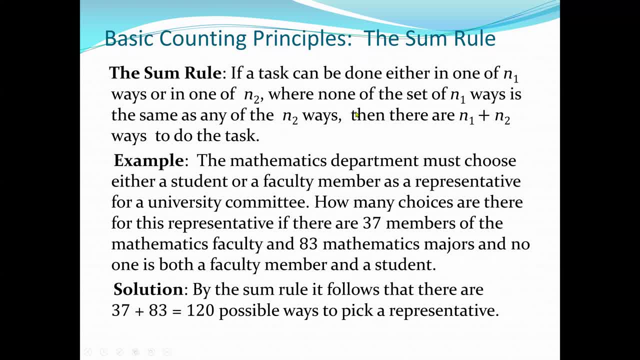 we are using the same dna sequence. we are using the same dna sequence here now we move to the sum rule now. so with the summary, we said that if a task can be done is the same as any of the N2 ways, So the two ways don't have to be the same. 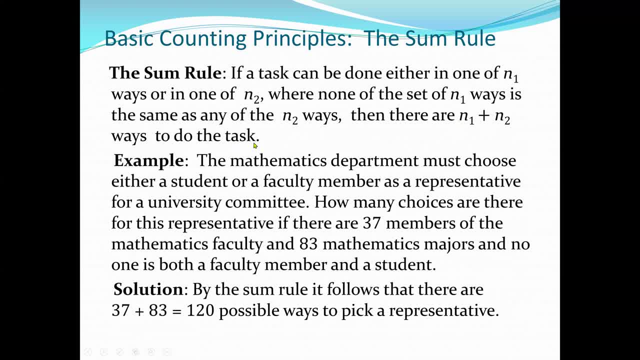 Then there are N1 plus N2 ways to do a task. The goal here we don't want to duplicate. If N1 and N2 have the same, we are doing one thing. We record it only once. So again, here we say if a task can be done either in one. 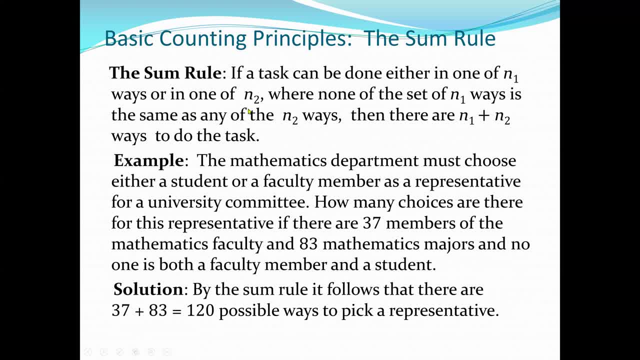 of the N1 ways or in one of the N2 ways. when none of the set of N1 ways is the same as any of the N2 ways, there's no duplicate. then there are N1 plus N2 ways to do the task. 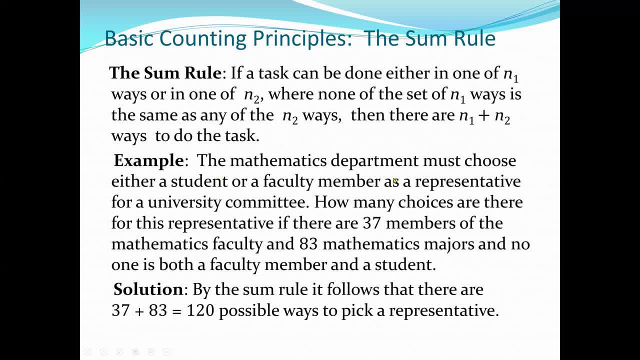 So example: here we have a mathematics department must choose either a student or a faculty member as a representative for university committee. So how many choices? How many choices are there if this representative, if there are 37 members of the faculty, mathematics faculty? 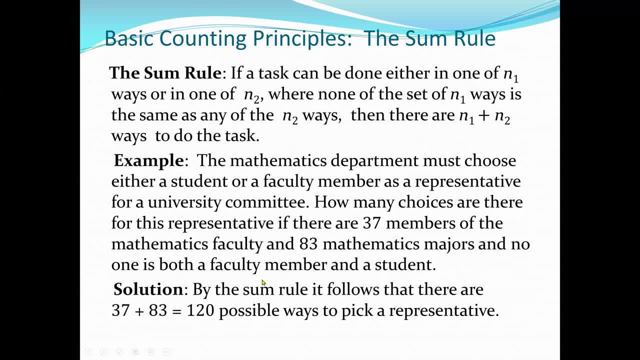 and 83 mathematics majors, and no one is both faculty member and a major. So this means again, the meeting or the representative for the university committee can be either a student or the faculty. Now we have 37 members of the faculty and 83 mathematics majors. 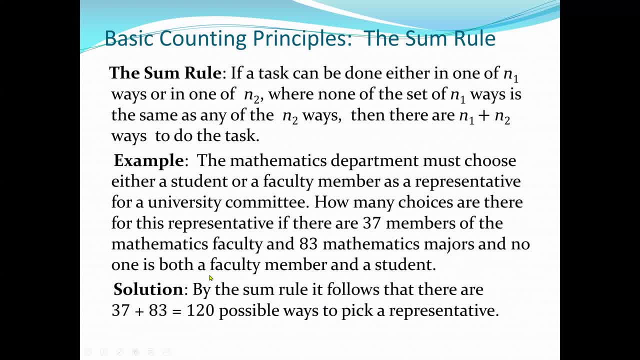 So we say by some rule, since here we say that, remember the rule- here we say that N1 way, N2 way, N1 way is the same as any of the N2 ways, None of them. So there's no duplicate. 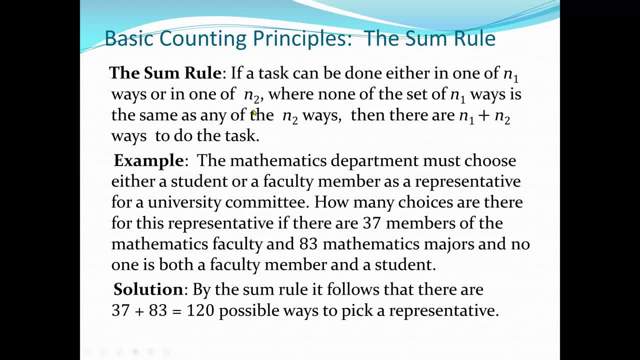 If a task can be done either in one of the N1 ways or N2 ways, where none of the set of N1 ways is the same as any of the N2 ways- there's no duplicate- then we can have the two. 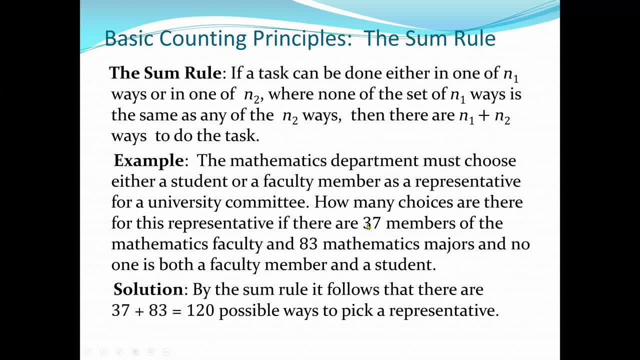 So the same thing. example here: we can see that we have 37 members of the mathematics faculty. We can see that we have 38 members of the mathematics faculty and 83 mathematics majors, but there's no one that is both mathematics faculty. 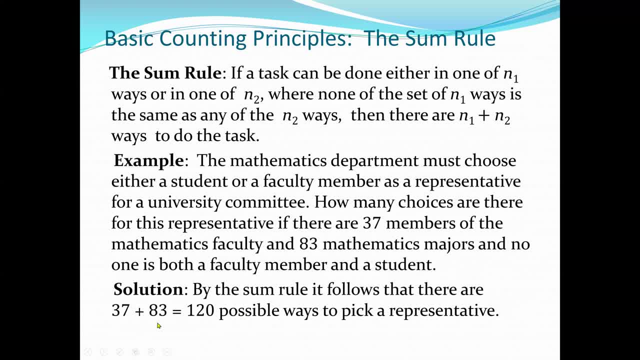 or student major. So if there's none, then we can just add a two, So the solution will be 37 plus 83.. Now if there is, we take only one, so we have to subtract intersection. 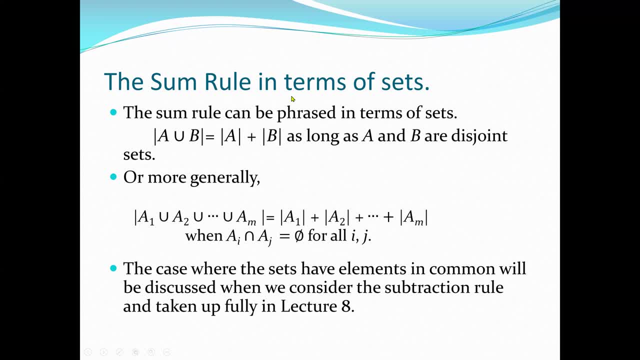 that's what we take as the sum rule. in terms of the set, we have a union. b means everything in a and everything in b, but not no duplicate. so the sum can be phrased as this then: 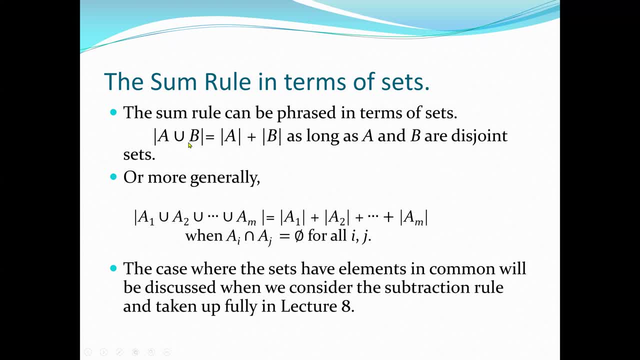 a union b, since there's no duplicate. and also we say when we are sami, there was, we don't had a duplicate, and that's why we're using the term as long as a and b are this joint. this joint means again, there's no duplicate, there's no intersection between a and b. so a1 union a2, all the way to. 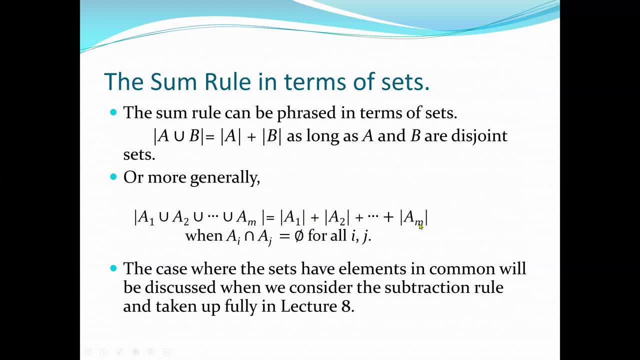 union am can be a1 plus a2 on the way to a. this is if they are disjoint and that's the statement here. ai, intercept, aj is equal to zero, which means intersection, means there's no duplicate. we don't have item that is in ai and also it's in aj. 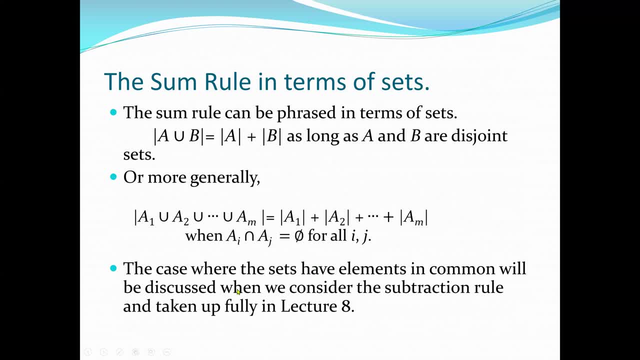 so the case where they said have element in common. we are going to discuss that one again in lecture number eight, which is unit eight. but what we normally do it is same as writing this general addition: if i have a union b equal to a plus b, then minus a intercept b, which means i'm taking a. 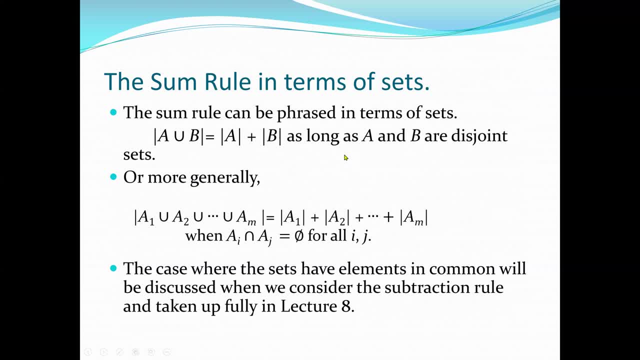 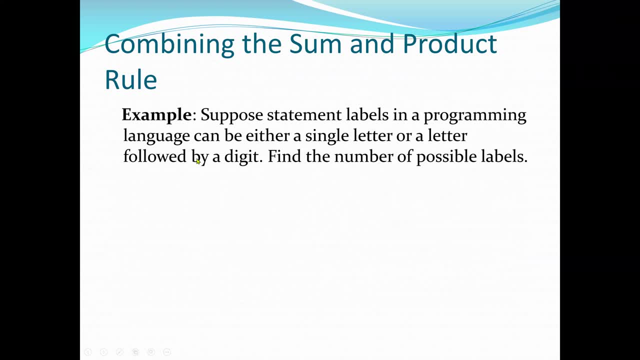 duplicate. if a and b are a case, then the interstate b will give us some value. so combining the sum and the product, we have an example. suppose a statement levels in the programming language can either be a single letter or a letter followed by a digit. find a number of possible labels. 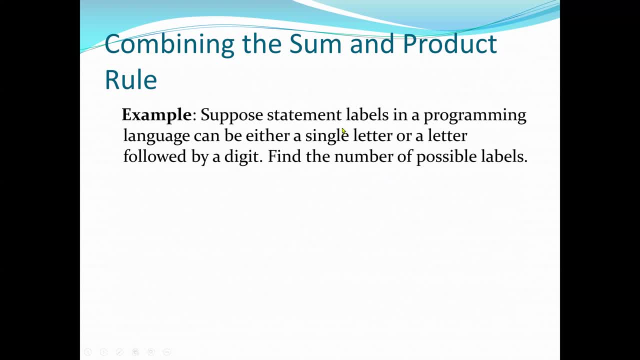 so suppose a statement labels in a programming language can be either a single letter or a letter followed by a digit. find a number of possible labels. so the solution will be: we use the product rule first. we use the product rule. so here we have 26 plus 26 times 10, which will give us again 286. 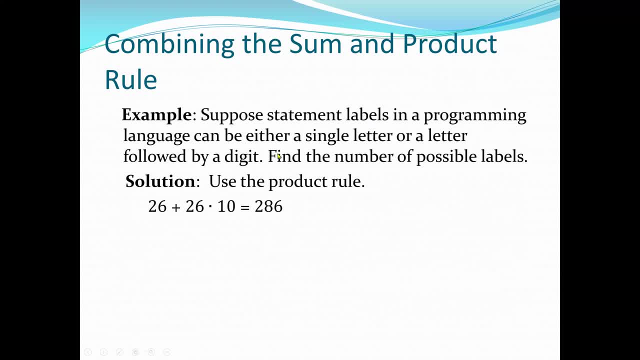 now the question is: suppose a statement label in a programming language can be either a single letter or a letter followed by a digit. so if it's a single letter, that's possible 26. next is a letter by a digit, so it's 26 times 10.. digit is from 0 to 9 or a letter. 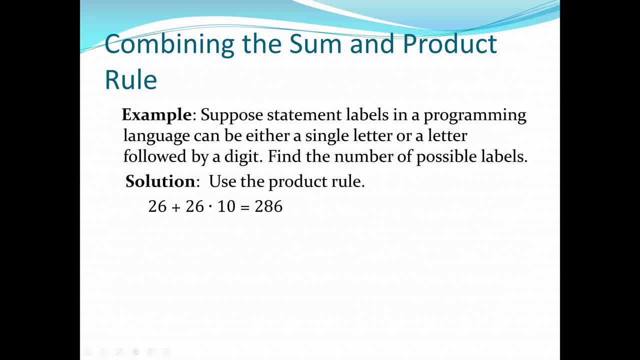 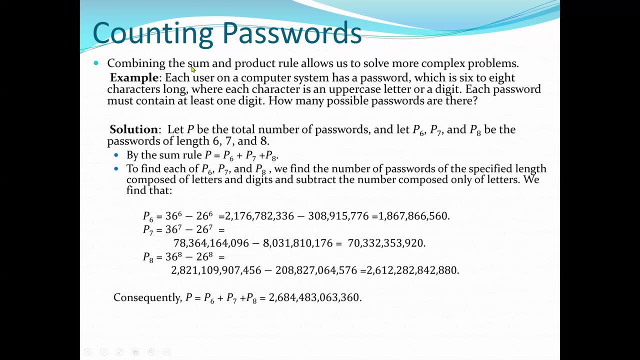 so that's why we have the 26, first because it's a letter and then next can be letter or a digit. 26 again the possible digit at 10, so 26 times 10.. also counting the password. here we say we can have a product rules also, which allow us to solve more complex problems. so example: 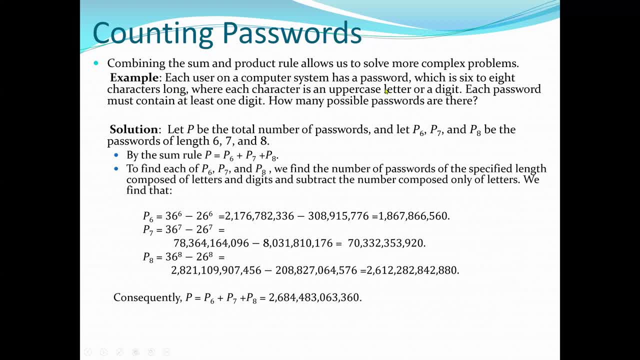 here we have. we say, each user on the computer system has a password which is six to eight characters long, where each character is an uppercase letter or a digit, and each password must contain at least one digit. how many possible passwords are there? so let's go back to the build tool again. we can see the possible. 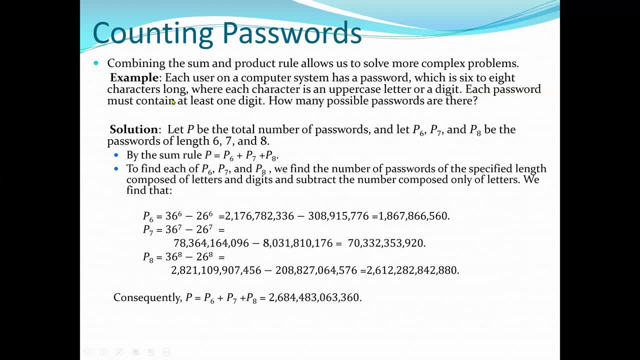 format of the password, which is again six to eight characters long, where each character is an uppercase letter or a digit. So here we say: let p be the total number of passwords, be the password of length from 6,, 7,, 8, because they say which is 6 to 8 characters long. 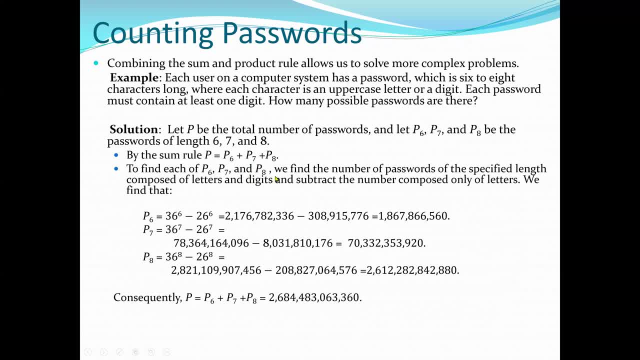 So by some rule, p can give us p6 plus p7 plus p8.. Now to find each p6, p7, p8, we need to find the number of passwords of a specified length composed of the letters and also the digits. Then we subtract the number of composed only of letters. So here we get. p6 gives us. 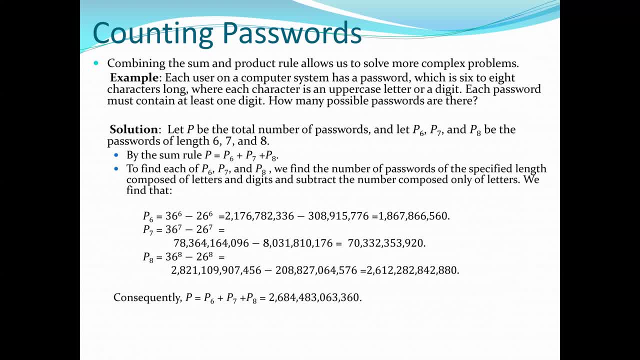 36 to the power 6 minus 26 to the power 6.. Remember, the lengths go up to 6.. And based on the question here, we say each user has a number of letters composed of letters. So each user composed. each user on the computer system has a password which is 6 to 8 characters. 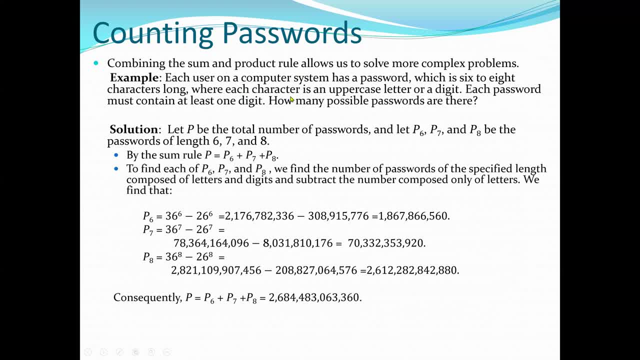 long, Then each character is composed of a letter or a digit. So that's why we have 36, because 26 characters and 10 digits, so 36.. 36 to the power 6, we did this because I have a possible digit and the character together is 36.. 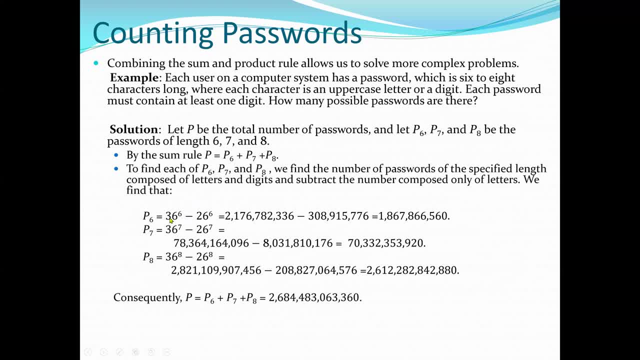 And the length is 6.. So to give me possible combination, give me 36 to the power 6.. But the question says: find p6, p7, p8. So just only the p6, p7, p8. So the possible 36 to 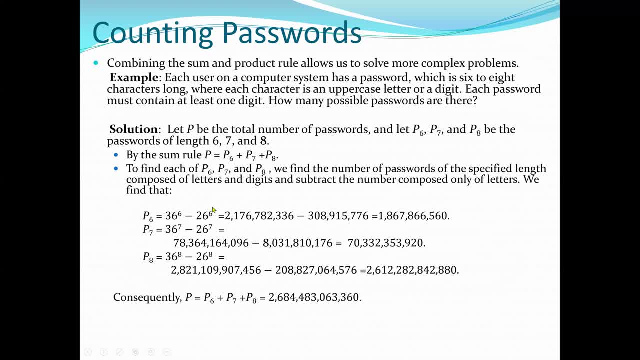 the power 6 minus 26 to the power 6.. And that will give us one point: almost 1.9 billion. Now for the seventh length: 36 to the power 7 minus 26 to the power 7.. Based on the question: 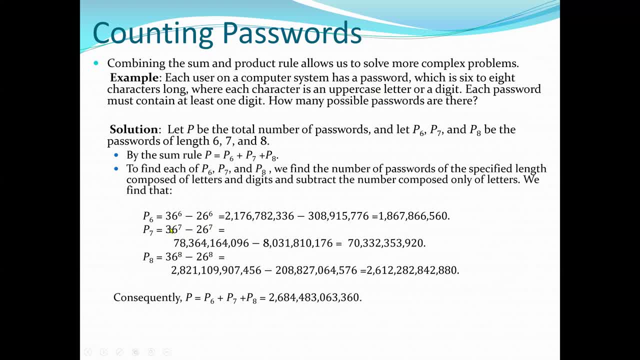 we are going to take the character out. So, plant, we have digits and character together, minus characters, And the lengths are the exponents. So length is 36 to the power 8 minus 26 to the power 8.. So the answer we got now we had all the length: p6,, p7,, p8. 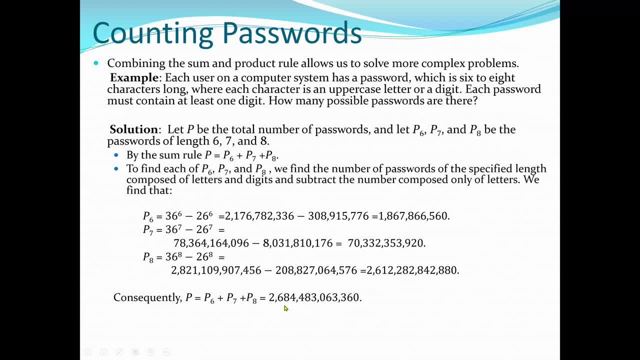 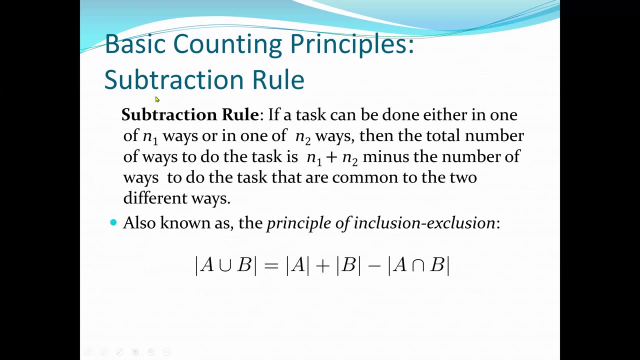 and that gave us two point six. that's a lot, almost trillion. I'll say two thousand six hundred eighty four billion. now, unless we move to the subtraction, we say that's a subtraction rule if a task can be done either in one of the n1 ways or 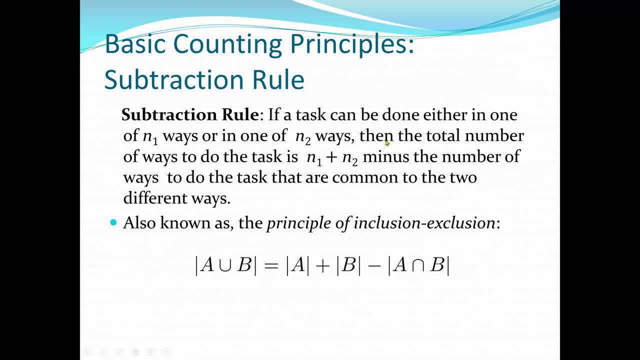 in one of the n2 ways, then the total number of ways to do the task is n1 and n2. one knows the number of ways to do the tasks that are common in the two different ways. so this is what we are saying, that we're going to discuss. if 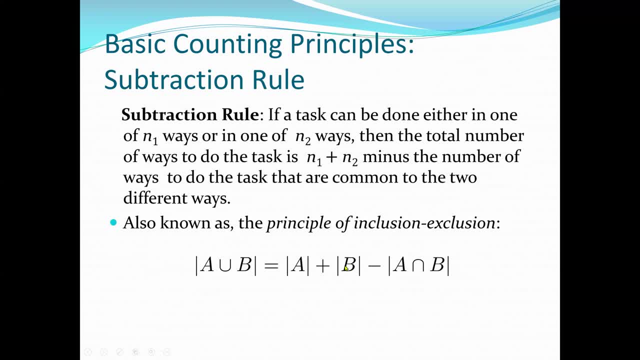 this: if our let's say this is a set a and b, if the set A and B is disjoint, it means A union B will be a plus B If it's not disjoint, which means there's a possible that we have some element that is in both A and B together. So in this case we have to subtract it, So A intersect B will. 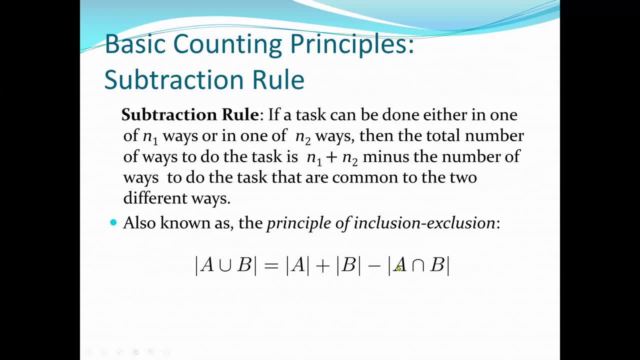 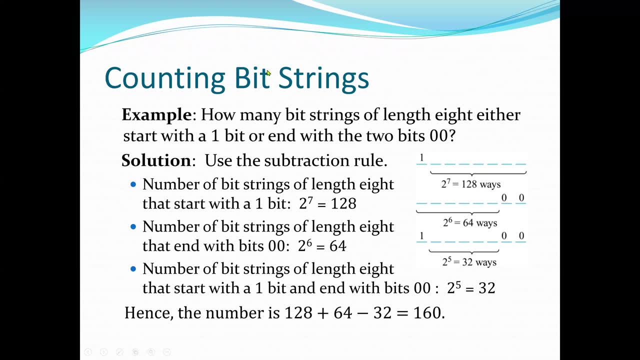 give us the number of element that is in common for both A and B when we subtract that out. So counting a bit strength, we have example here- say how many bit strengths of length either eight. how many bit strengths of length eight either start with one bit or end with. 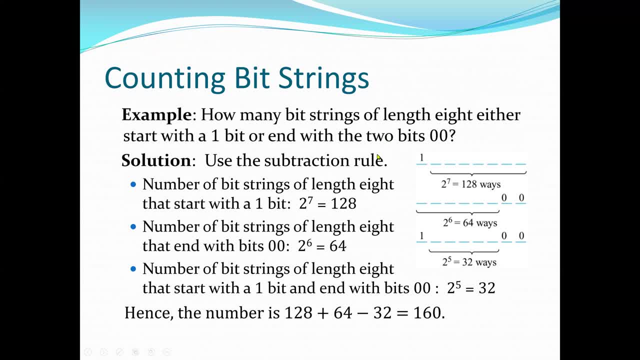 two bits. So you start with one with a one bit, or it end with the two bits, zero, zero. So the solution here I'm going to use the subtraction rule. First, the number of bits of length eight that start with one bit is two to the power seven. 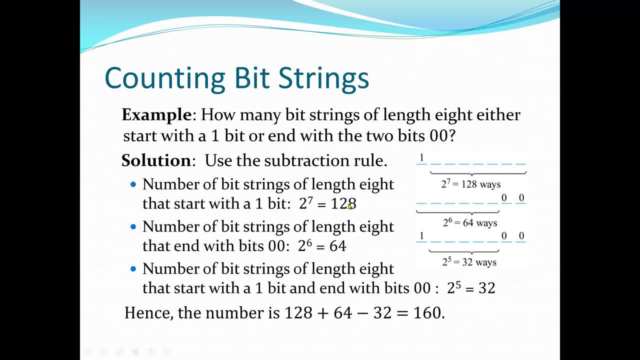 Which will give us 128.. Now the number of bits of length eight that end with a bit zero, zero will be two to the power six, which is 64.. Then the number of bit strengths of length eight that start with one bit and end with zero, zero will be two to the power five. 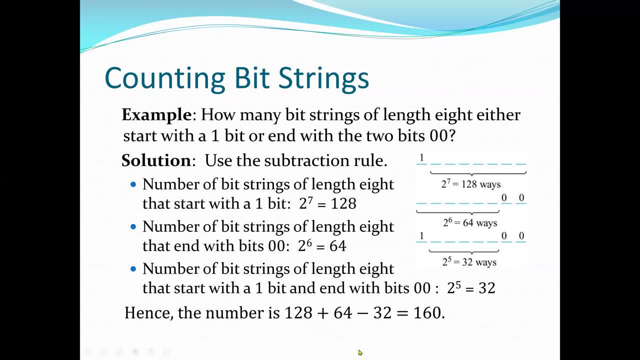 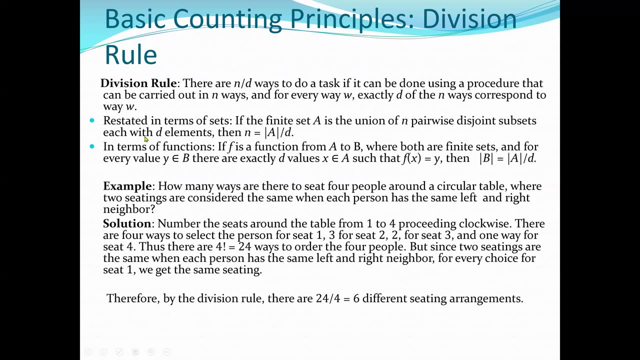 which is 32.. So in total we get 128 plus 64, then minus 32.. So also we have the basic counting principle for division rule, And here we are saying that there are n by 10 or n divided by 10. 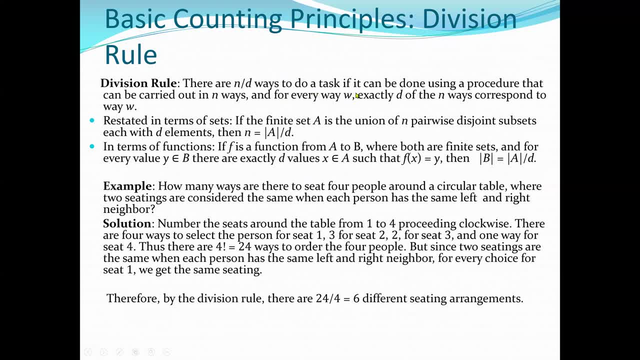 ways to do a task if it can be done using the procedure, that can be carried out in n ways And for every way w. exactly d of the n ways correspond to way w. We can restate in terms of sets. So we can say that if affinity set A is the union of 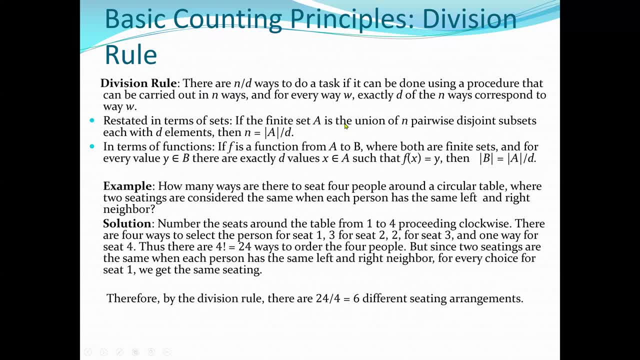 n pairwise disjoint subsets, each with d element, then n will give us absolute A divided by d. Then in terms of function we can say that if f is a function from A to B where both are finite sets And for every value y belongs to B, there are certainly d values of s belongs to A. such, 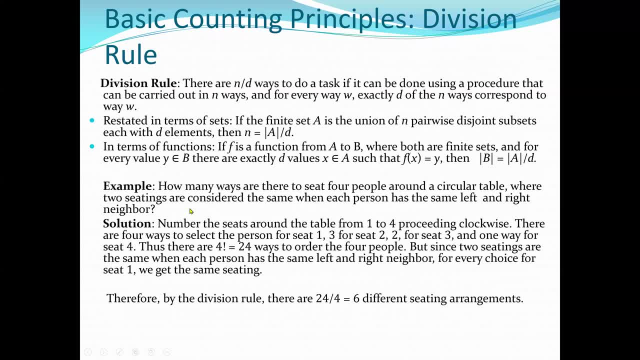 that f at s equal to y, then B will give me A divided by d or absolute A divided by d, And that's again division rule. Now let's see example: how many ways are there to sit four people around a circular table? 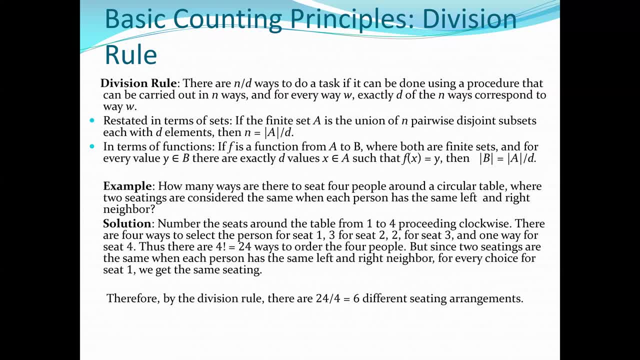 Let's see. Well, two sittings are considered the same when each person has the same left and right neighbours. So to number the seats around the table from one to four, proceeding clockwise, and then there are four ways to select a person for seat one, three, four. seat two, three, four. 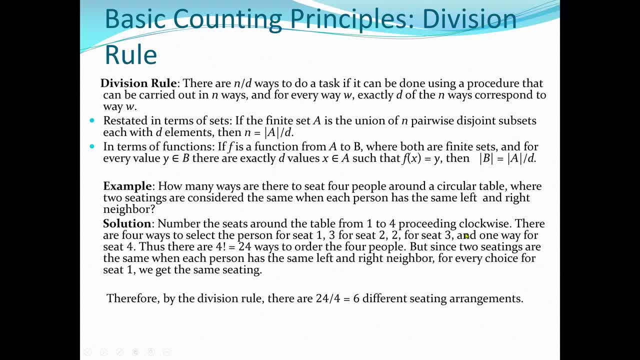 seven, six And two for seat three, And also we have one way for seat four. Therefore, here we are going to get four factorial, which is 24 ways to order the four people. But since, again, two sittings are the same, 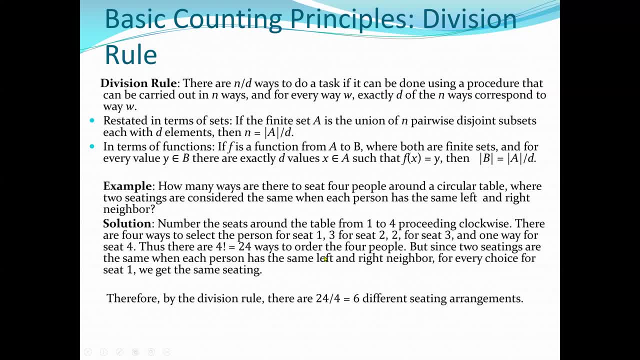 when each person has the same left and right neighbor, we can say that for every choice for seat one we get the same seating. Therefore, by division rule, there are 24 by four, which is six different seating arrangements. So the last section will be the tree diagrams. 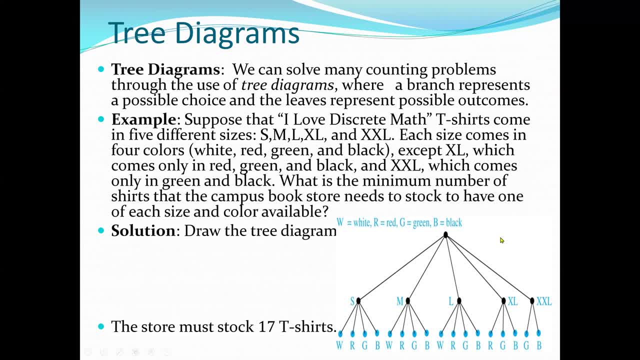 Tree diagrams are also we can use for counting a lot. We can say: we have the root, which is one. Normally the root of a tree is at the top in computer science. Then from the root we branch to five different places. 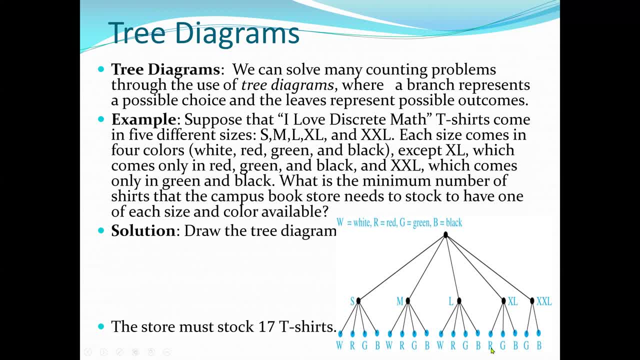 Then from there we get our outcome, which will be our leaves. So we can count the number of nodes we have per level. The number of nodes are the dots And this is called the root node. So you can use- you can also use this to count on items- 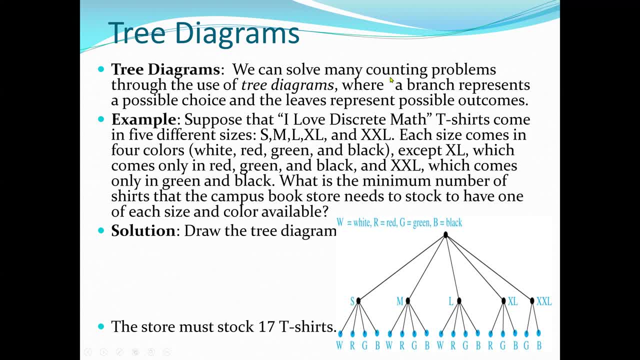 So let's say, for example, here we say we can solve many counting problems, So we can write, for example, a queen number. You can write a number, you can also do a number of nodes. you can add a number of numbers, and then you can add a number of numbers. 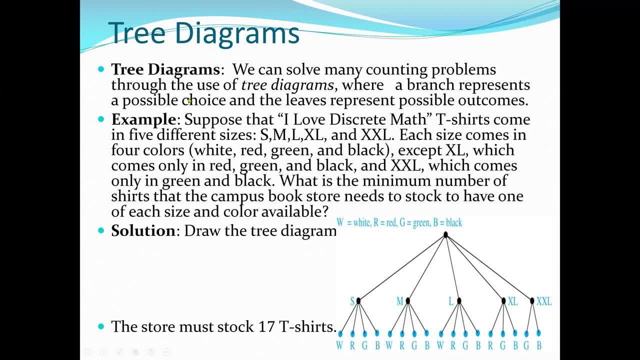 That's where we get the key. So by dividing by two, by divided by two, we can say we are able to solve many planning problems, even when we have to divide by two. So that's where we get, I think, three. 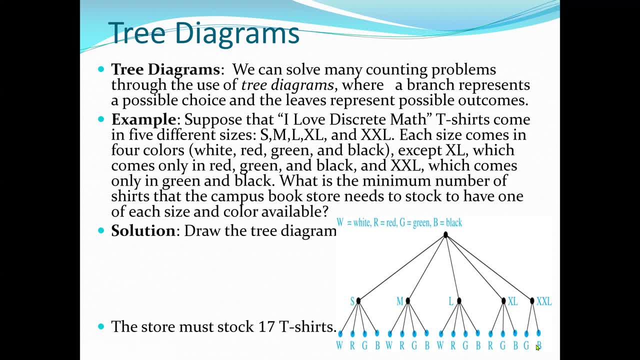 That's where we can go more and we're able to solve a lot of problems. And we're able to solve problems. So, again, a branch represents a possible choice And the leaves represent possible outcome. So the leaves, at the end, when we have GB, GB, their branch will be our edges. 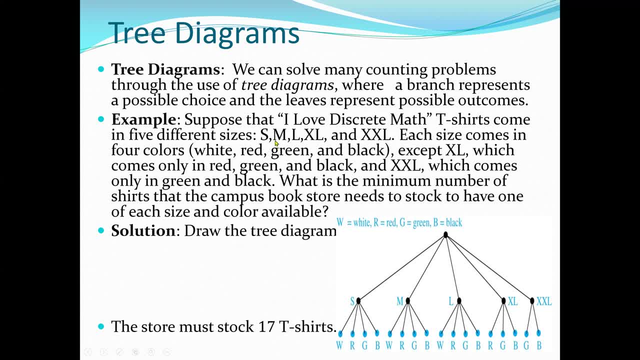 where we branch to go. So we have example here. Suppose that I love discrete math, shirts come in five different sizes. so i have a t-shirt that come in five different sizes. each size comes in four colors. i said sl, which comes only in three colors, and ssl. 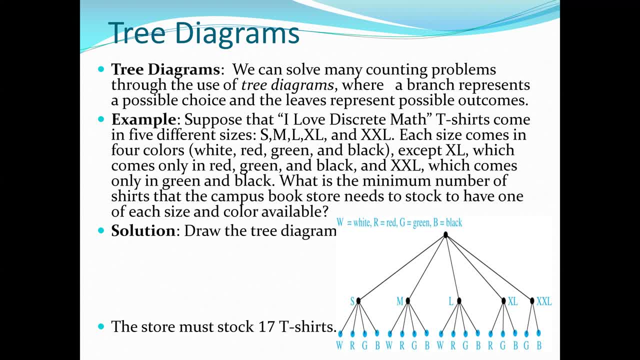 which comes only in green and black. now the question said: what is the minimum number of shares that the campus bookstore needs to install to have one of each size and a color available? so here we use a tree diagram to solve this program, which is very good because we start from the root and we can see that we have small, medium, large, sl and ssl. 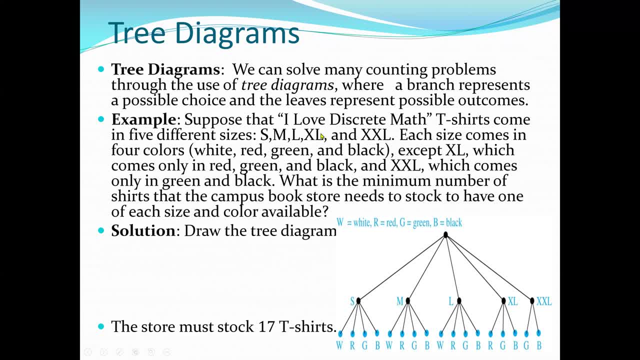 but according to the question- i think the small for the this critique- come in five different sizes. which size come in four colors? so we have white, red, green and black, a set sl which comes only in red and green and black. so when you look at sl leaf we have only 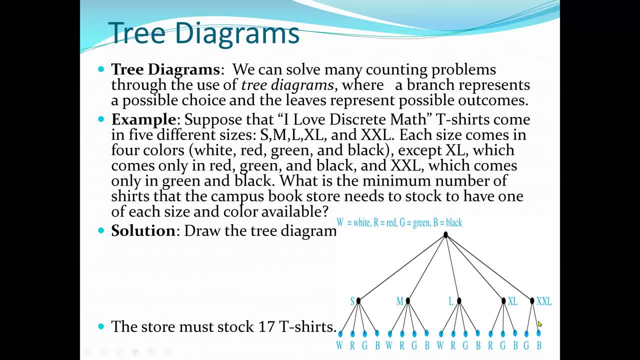 red, green, black, ssl, camberley, green and black, which is the condition? green and black, ssl and the large, small, medium large have all the four colors. now the question. so what is the minimum number of shirts that the simplistic bookstore needs to stop to harvest? so the minimum would be the down here. if we had one, two, three, four, five. 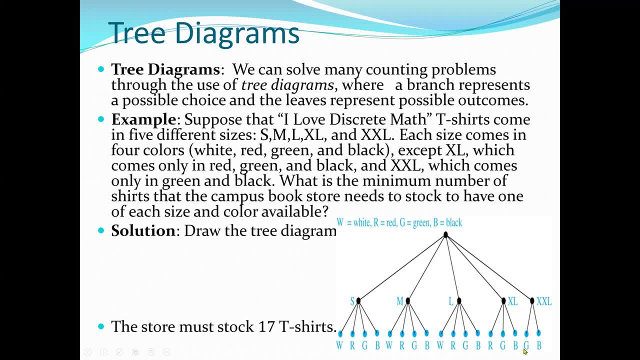 six, seven, eight, nine, ten, eleven, twelve, thirteen, 14, 15, 16, 17.. so the answer will be 17.. and we saw this problem using the. it's a kind of product rule, but we are using the tree structure. we start with the root, which is only one, and the condition of the question is based on the sizes. so we say, if 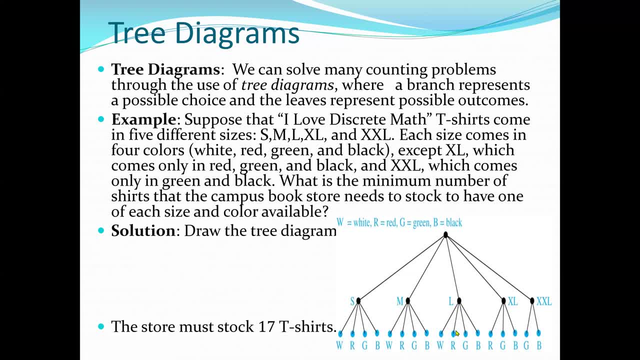 you are small, medium and large, you have all the four possible colors. if your sl and ssl, there's limited color. so sl is three different colors and ssl is only two different colors. so that's why we have ssl2, sl3 and the rest are four. so we had all the least values and that give. 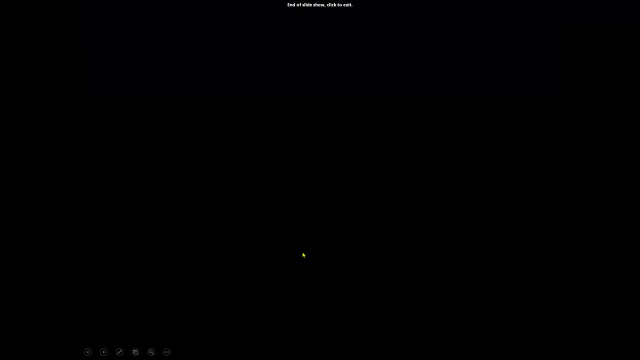 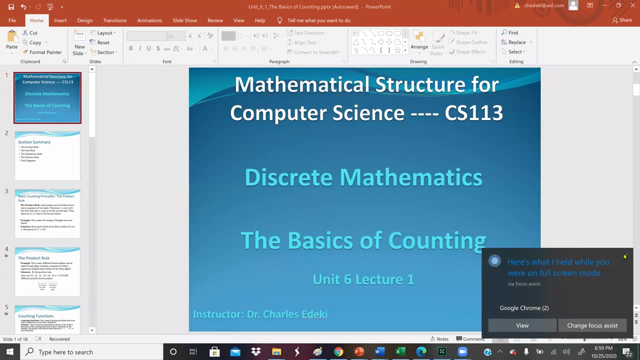 us 17.. so this will be the conclusion of our unit 6-1 lectures and again, if you have any question about the assignment, please feel free to ask me in the comment section below. if you have any questions about the assignment, please feel free to ask me in the comment section below. if you have any questions. 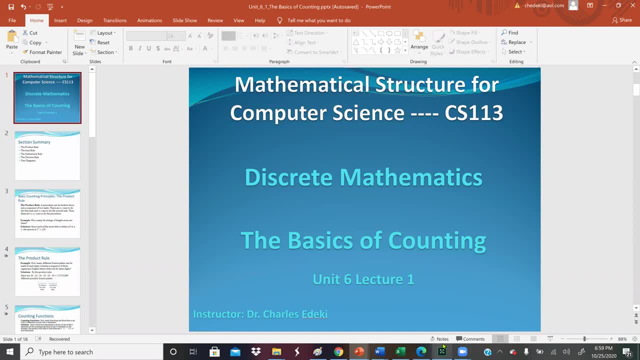 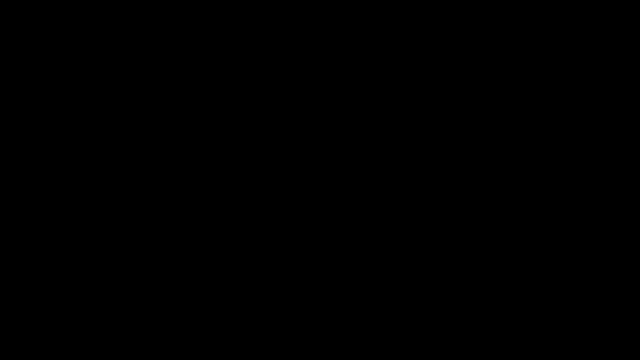 about the assignment. please feel free to ask me in the comment section below if you have any question about the assignment. please feel free to ask me in the comment section below. if you have any question, you can send an email. so again, wish everybody the best and thank you for your time. 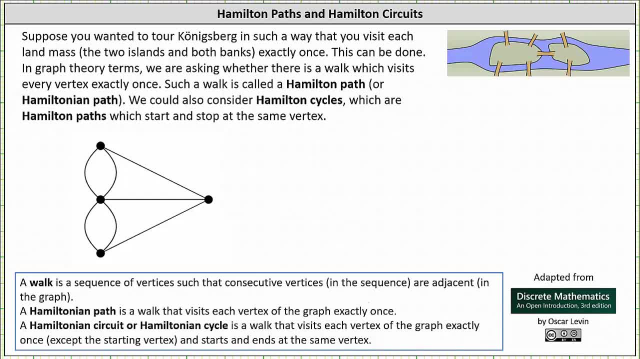 Welcome to a lesson on Hamilton paths and Hamilton circuits. Let's begin by revisiting the graph for the seven bridges of Konigsberg problem shown below. Recall: each vertex represents a landmass and each edge represents a bridge. Suppose you wanted to tour Konigsberg in such a way that you 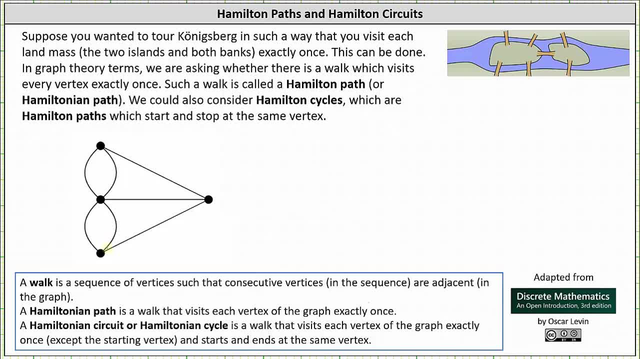 visit each landmass exactly once. This can be done In graph theory terms. we are asking whether there is a walk which visits every vertex exactly once. Such a walk is called a Hamilton path or Hamiltonian path. We can also consider Hamilton cycles or Hamilton circuits, which are Hamilton. 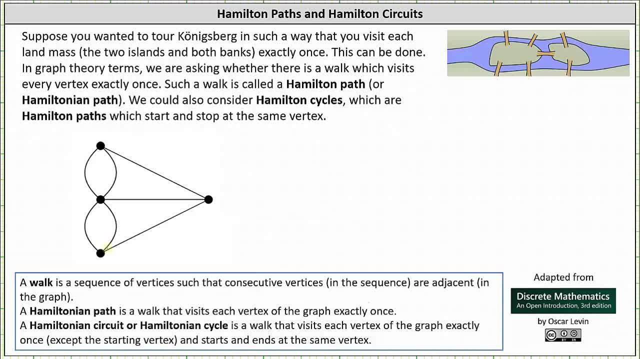 paths which start and stop or start and end at the same vertex. Recall that a walk is a sequence of vertices such that consecutive vertices in the sequence are adjacent in the graph. And again, a Hamilton path or Hamiltonian path is a walk that visits each vertex of the graph.